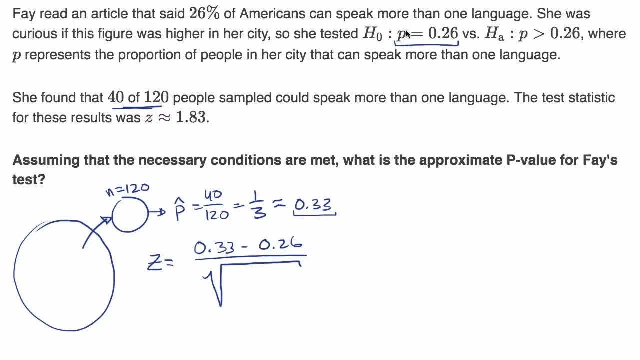 And we've seen that in previous videos. That is just going to be the assumed proportion, so it would be just this: It would be the assumed population proportion times one minus the assumed population proportion over n. In this particular situation, that would be 0.26 times one minus 0.26,. 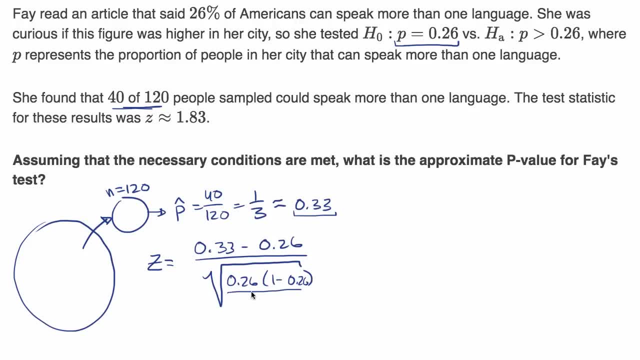 all of that over our n, That's our sample size, 120.. And if you calculate this, this should give us approximately 1.83.. So they did all of that for us. And they say: assuming that the necessary conditions are met. they're talking about the necessary conditions. 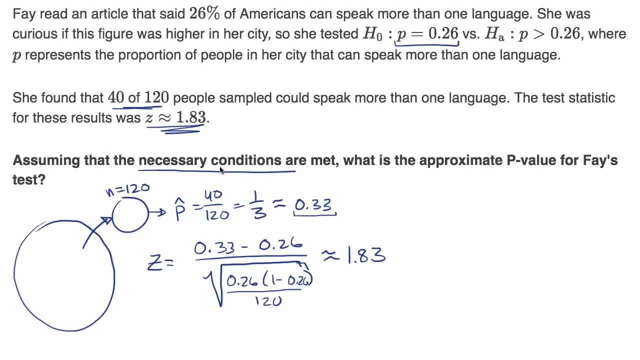 and they're talking about the necessary conditions to assume that the sampling distribution of the sample proportions is roughly normal, And that's the random condition, the normal condition, the independence condition that we have talked about in the past. What is the approximate p-value? 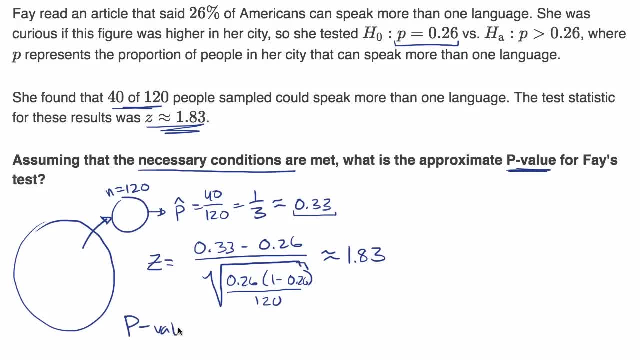 Well, this p-value- this is the p-value- would be equal to the probability of in a normal distribution. we're assuming that the sampling distribution is normal because we met the necessary conditions. So in a normal distribution, what is the probability of? 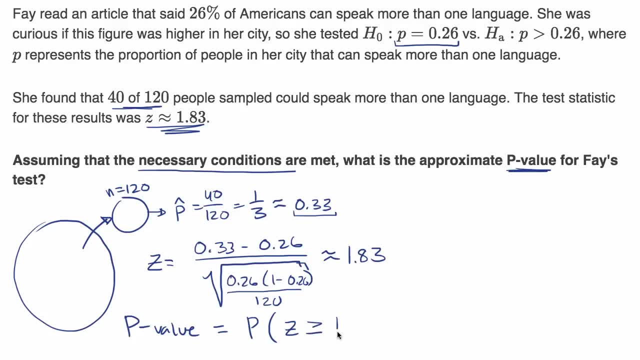 in a normal distribution, what is the probability of? what is the probability of getting a z greater than or equal to 1.83?? So to help us visualize this imagine, let's visualize what the sampling distribution would look like. We're assuming it is roughly normal. 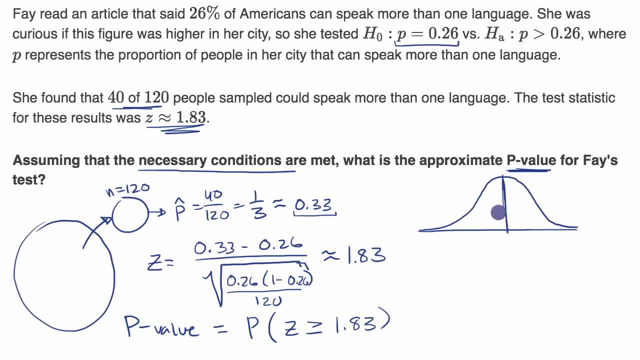 The mean of the sampling distribution right over here would be the assumed population proportion. So that would be p-naught when we put that little zero there. that means the assumed population proportion from the null hypothesis and that's 0.26.. 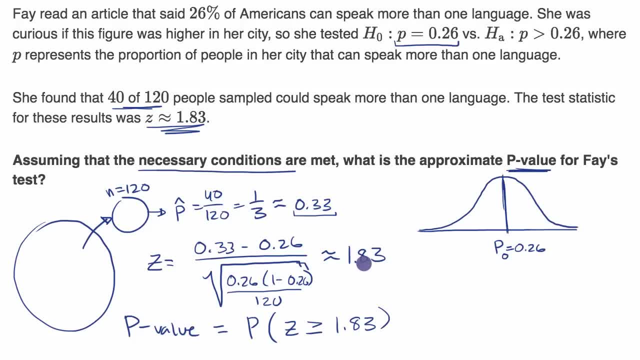 And this result that we got from our sample is 1.83 standard deviations above the mean of the sampling distribution, so 1.83.. So that would be 1.83 standard deviations, And so what we want to do, this probability is this area. 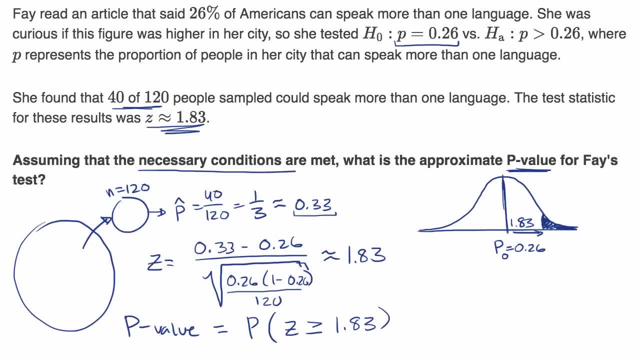 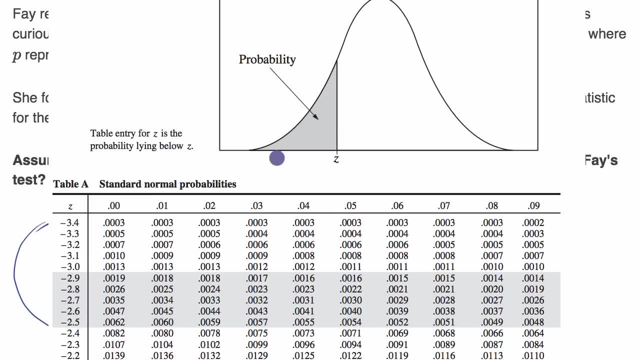 under our normal curve right over here. So now let's get our z-table. So notice, this z-table gives us the area to the left of a certain z-value. We wanted it to the right. We wanted it to the right of a certain z-value. 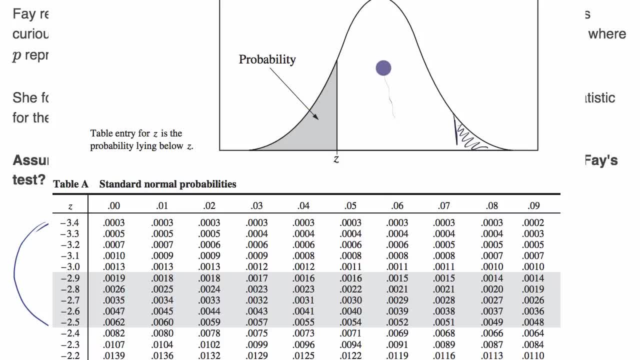 But a normal distribution is symmetric, so instead of saying anything greater than or equal to 1.83 standard deviations above the mean, we could say anything less than or equal to 1.83 standard deviations below the mean. So this is negative 1.83.. 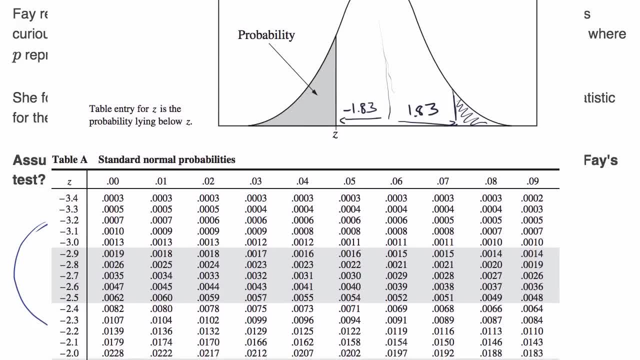 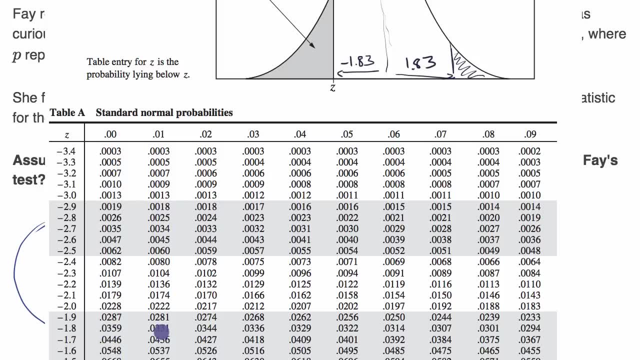 And so we could look at that on this z-table right over here. Negative one, let me, negative 1.8, negative 1.83.. And so 1.83 is this right over here, So 0.0336,. so there we have it. 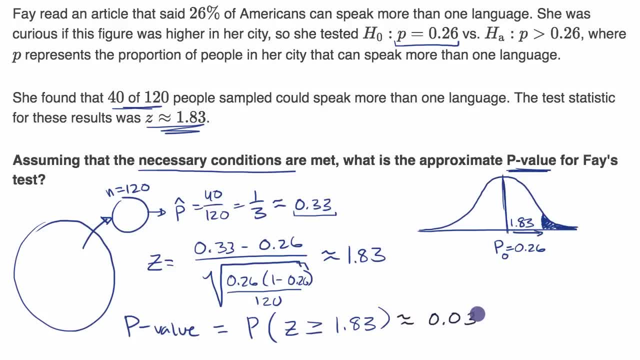 So this is approximately 0.0336, or a little over three percent, or a little less than four, And so what Faye would then do is compare that to the significance level that she should've set before conducting this significance test. And so for significance level. 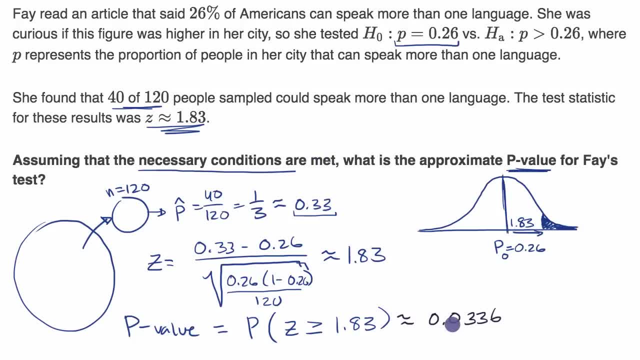 was, say, 5%. well then, in that situation, since this is lower than that significance level, she would be able to reject the null hypothesis. She would say, hey, the probability of getting this result, assuming that the null hypothesis is true. 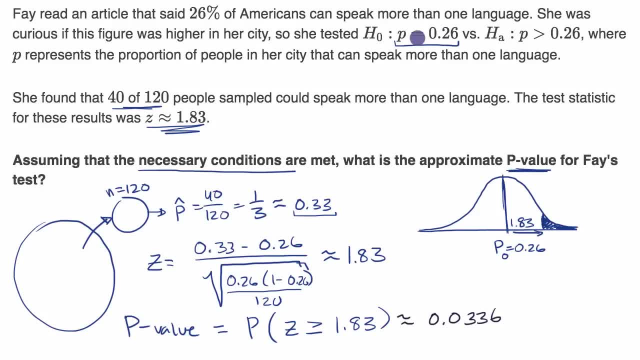 is below my threshold. it's quite low, and so I will reject it, and it would suggest the alternative. However, if her significance level was lower than this, for whatever reason, if she had, say, a 1% significance level,